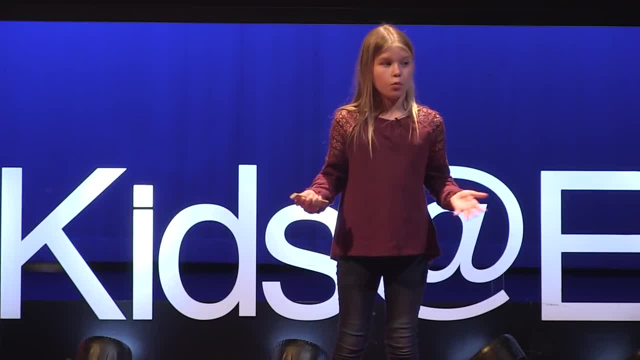 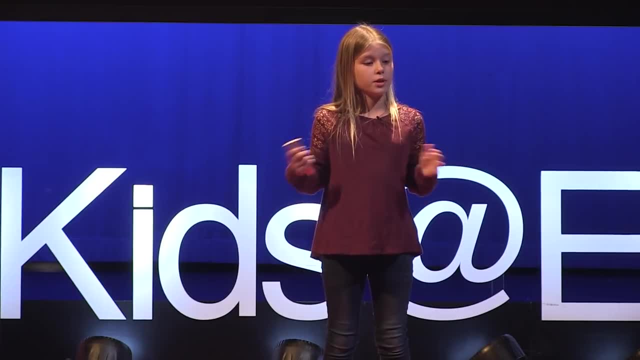 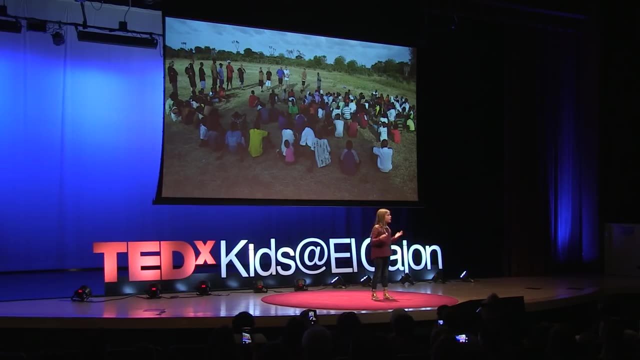 go to school every day. 25 million of them will never go to school, either because of money or there isn't a school in the area. Most of the kids that aren't able to go to school are girls. One of the worst places for school is Africa, because 33 million kids 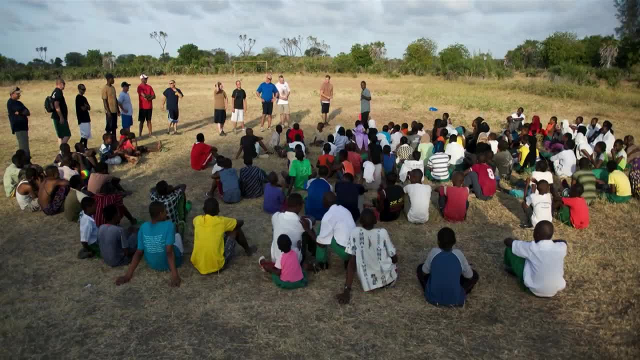 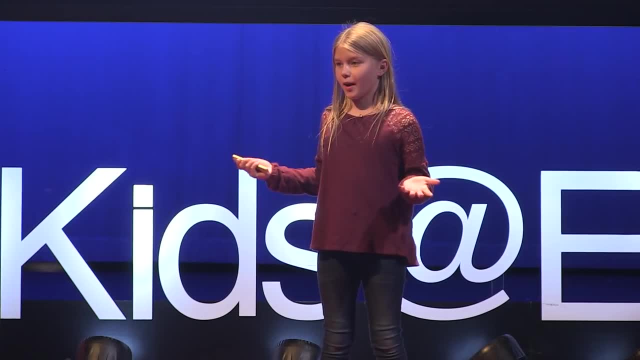 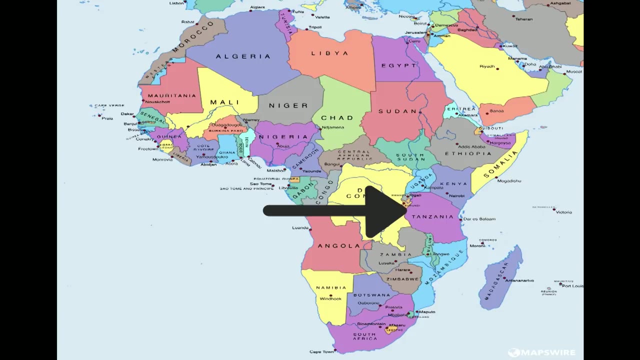 can't go to school there, and 18 million of these are girls. Only two-thirds of these kids will ever graduate high school. This is an amazing story about a girl named Jacinta at the age of 13.. She lived in Tanzania, a country in Africa, when 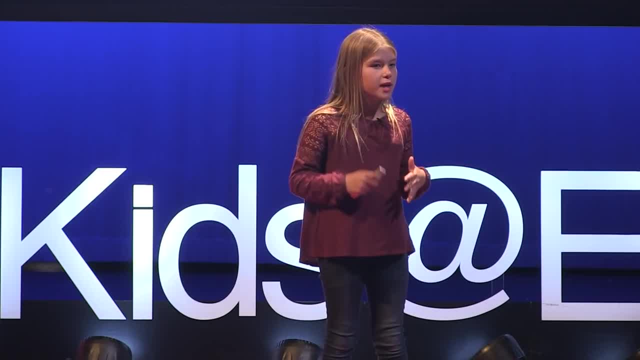 her family could no longer afford for her to go to school, so she had to drop out. She then had to work as a servant 18 hours a day and only made $13 a month. Then a charity called CAMFED raised money for her to go to school, and she was able to go to school for. 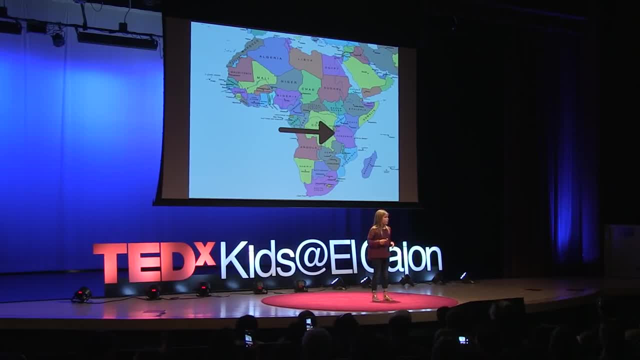 Jacinta and her family, so that she would not have to work anymore and could go back to school. Later she was sent home and had the opportunity to start school once again, so she headed back to school. After she went to school she got a great job and was able. 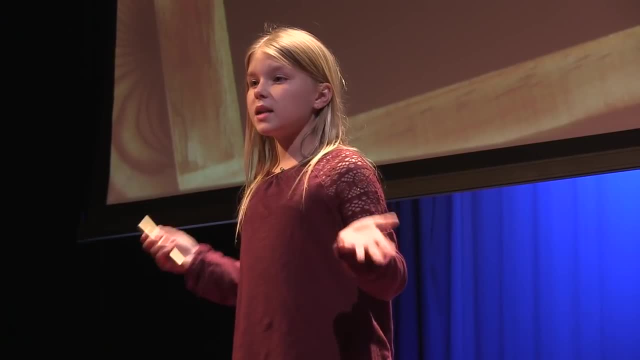 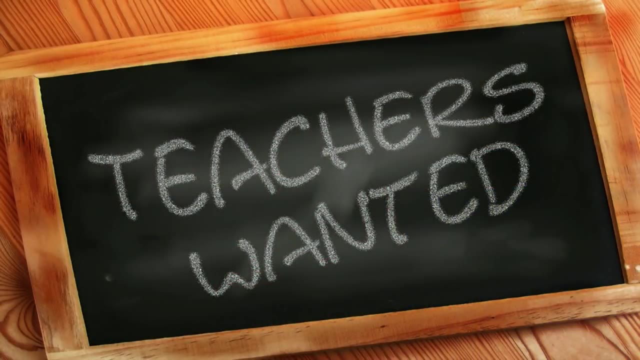 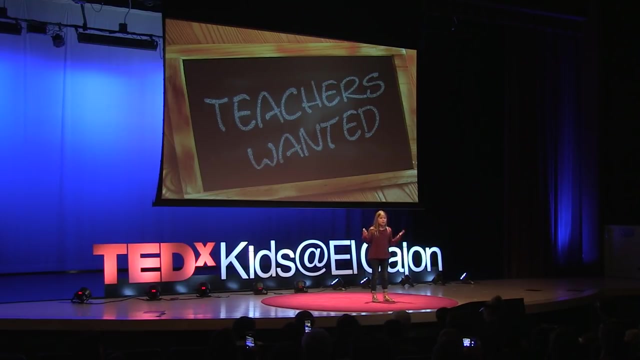 to send her brothers and sisters to school. But it's not just the kids and families that don't have enough money, it's there's not enough teachers. For example, in India they need about 350,000 workers And in West Africa they need about 380,000 more teachers. But for every kid in the world, 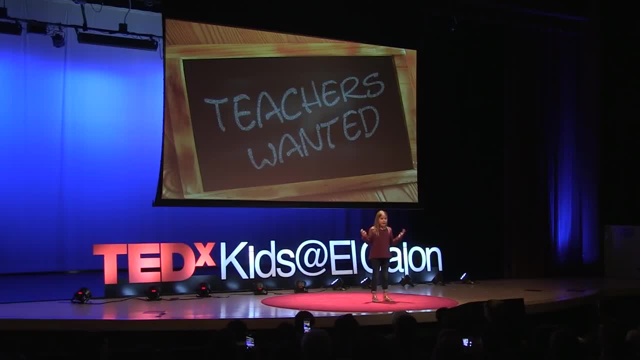 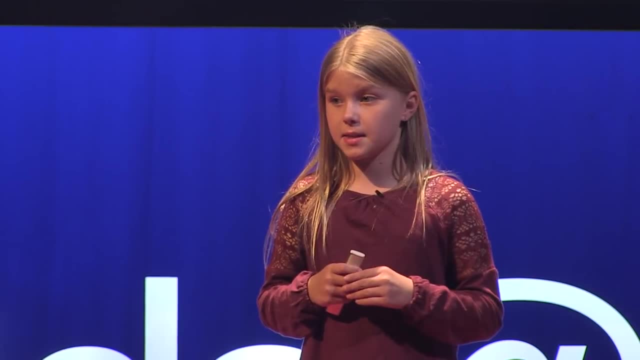 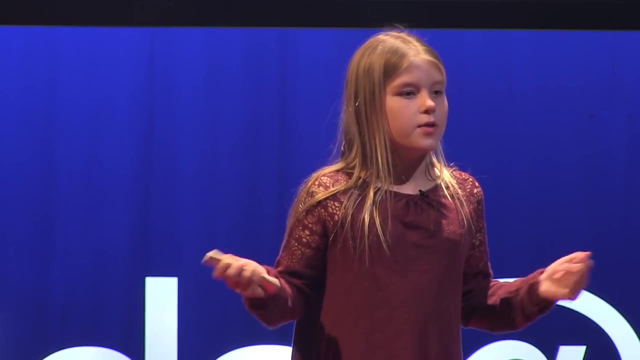 to be educated. we would need approximately 5 million more teachers. When adults don't get proper education as kids, it leads to bad things. For example, if you aren't literate, you can't get a job, And if you can't get a job, you can't make any money. There's about 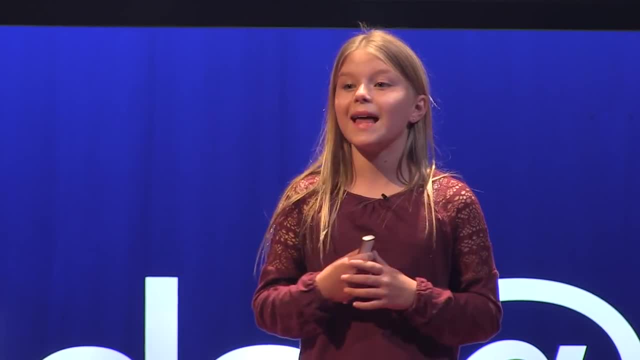 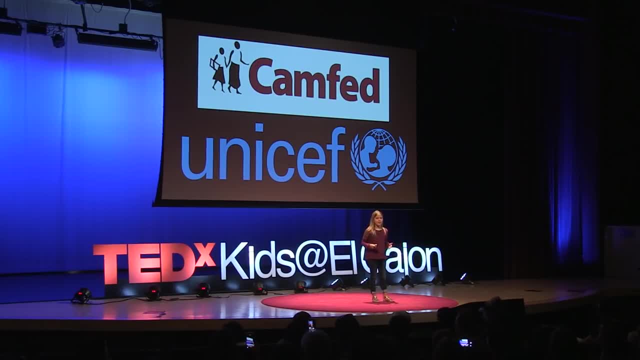 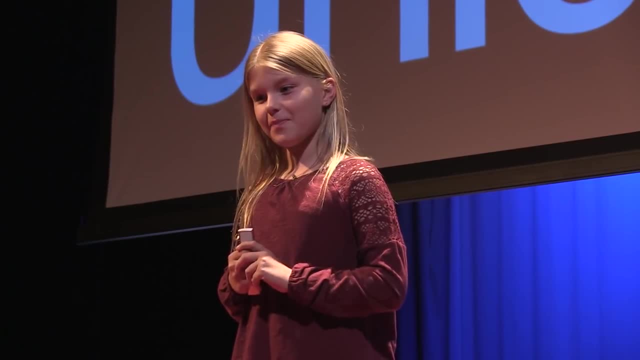 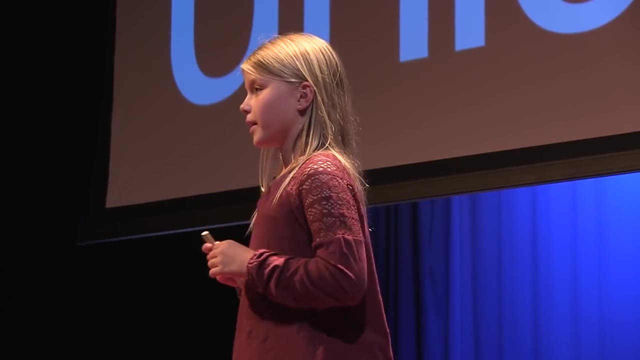 or writing. Some ways that you can help is by donating to a charity, as in UNICEF or CAMFED. CAMFED is a charity that helps girls in Africa go to school, while UNICEF is a charity that helps kids all over the world. But what would really help is spread the word, Tell your